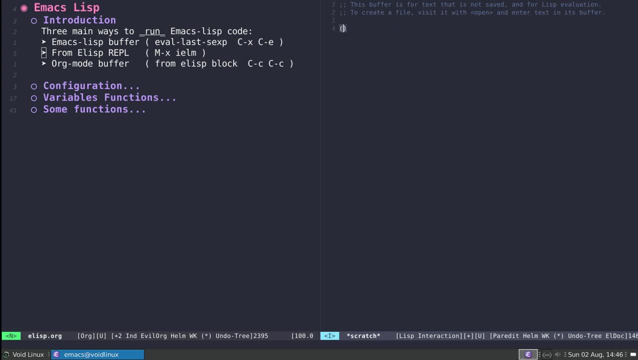 automatically inserts the corresponding parentheses. So this is very nice behavior again and I'll show you how to do it. I don't know how to explain this, how to kind of use this in a while, but let's say that I want to kind of print. 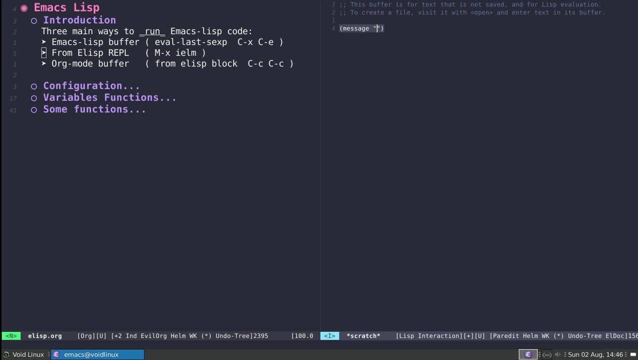 something to the echo area. You already know that I have a function for that which is called message, and this is printed to the echo area is going to be the string that I want to print Now to evaluate this inside of a Lisp, inside of a Lisp mode buffer. I can go to the end. 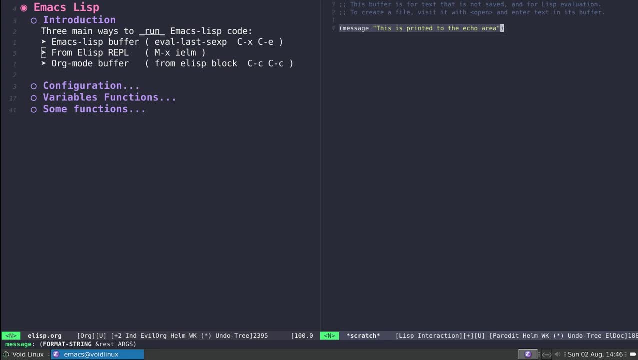 of the expression. and it is important that I go to the end because the command that I use is evaluate last expression, which is bound to control x, control e, And this evaluates again the last expression before the cursor. So I do need to go to the this. 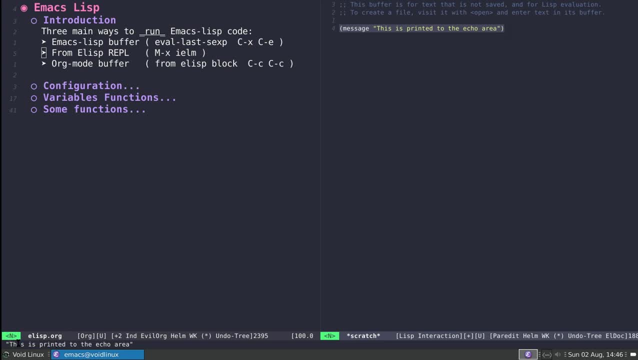 last parentheses here to the left and notice that I get the output. If I were to kind of use this command in the middle of the of the line, you notice that I get a Lisp error because this is a void variable again. So it's trying to treat this as a variable because it doesn't understand. 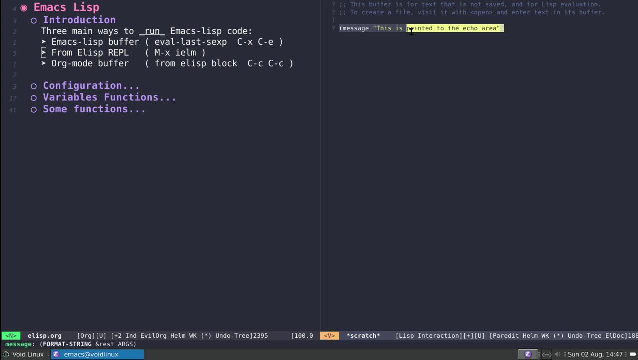 again that I have more stuff to come after the cursor. This is one way to run Lisp code. You also have ILM, which is essentially the ELISP REPL, so that is built into into kind of Emacs, meta x, ilm and you get the same environment. So par edit also works here. so I get the corresponding parentheses. 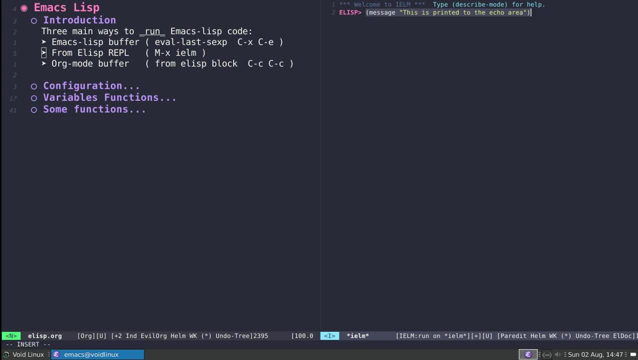 and except that it's kind of laggy. so this is not replay removing them, But let's try running the message function from here and you notice that I get the return value, which is the string, but I also get the side effect, which is big things being printed to the echo area. So I'm going to go. 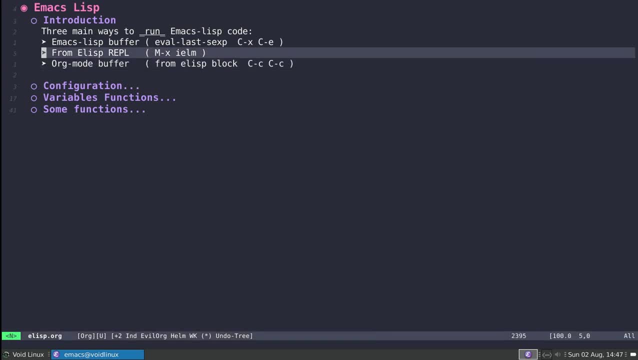 to the echo area. A third way of doing this is by using a org mode buffer. so we already saw that you can define source code inside of orgnode by using this, and then, if I set it to Emacs Lisp, I can type in something. so the same thing, For example, message this- gets printed, except that 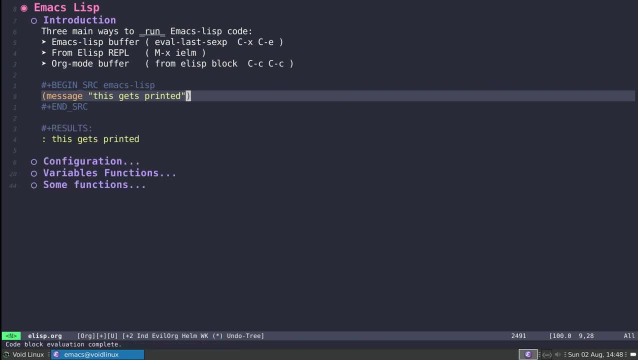 you notice that if I use ctrl c- ctrl c to execute here, this does not. I don't get the side effects. what only I that? the only thing that I get is kind of the, the return value. So this is the return return value for that. it happens that on the case of the message statement, it not only returns the 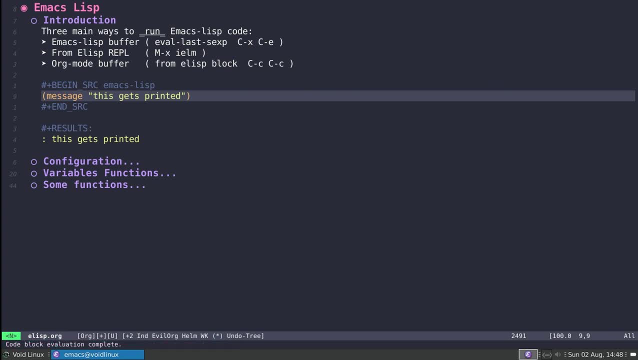 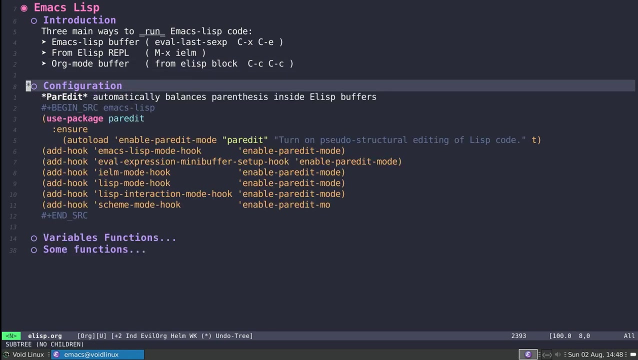 string, but it also prints the string to the echo area. you notice that i don't get anything printed down here, but i do get the, the return value. we'll be kind of doing a mixture of both. i'll be trying to show this from one org buffer so that it's easier to follow along. now regarding configuration. 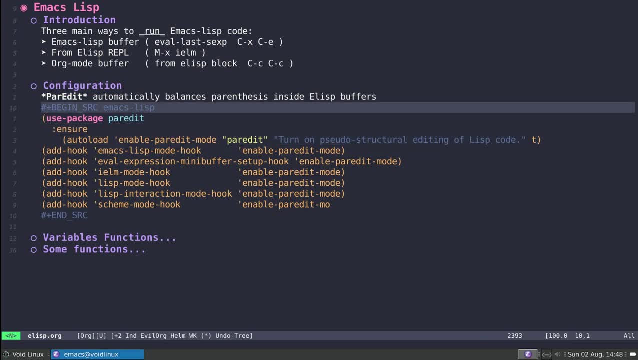 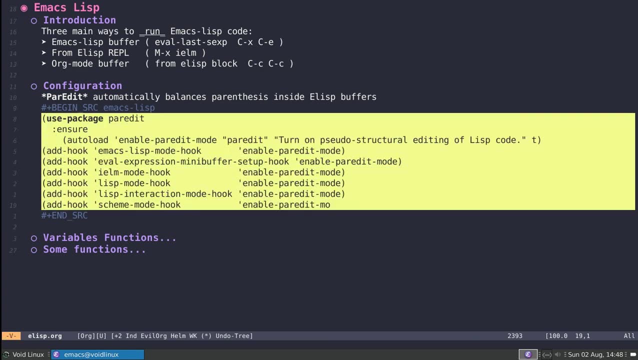 this, uh, the behavior that gets my kind of, uh, that nice behavior with the automatic, uh, balancing of parentheses is done by par edit. so this is the snippet of code. this is also on my github, so you can just clone the repo and it's going to be under. i mean, i can even show you. 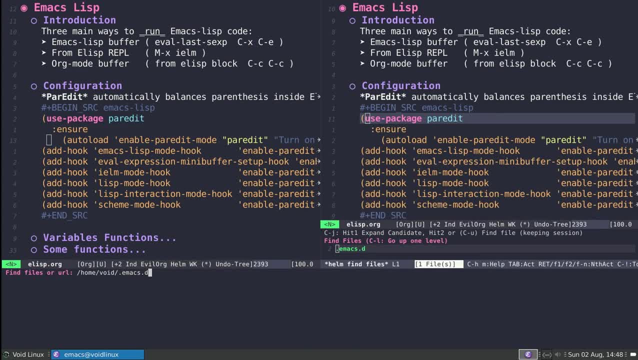 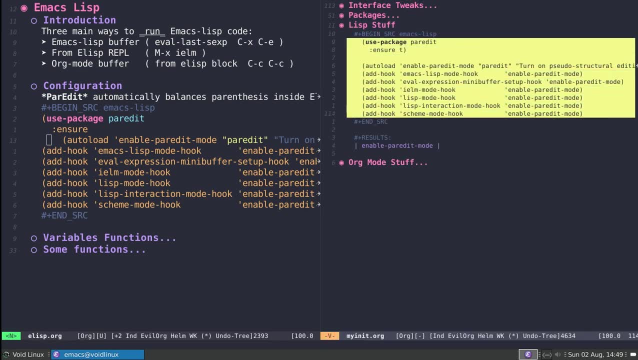 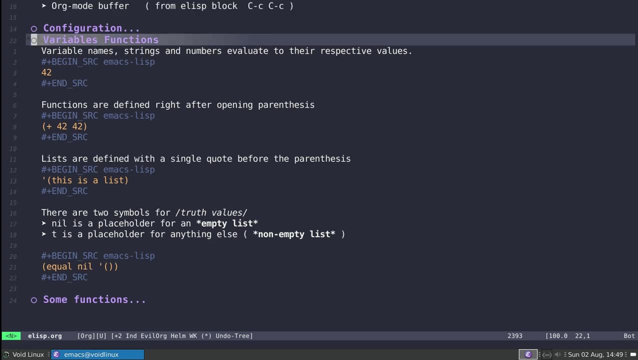 it's going to be under dot emacsd, my initorg it's going to be under lisp stuff. so if you want, you can just copy this piece of code here and you're all set because it's on this table. so let's talk a little bit about what we'll do. 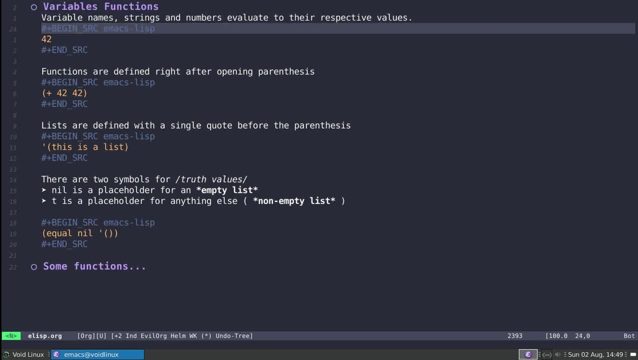 with regards to variables and functions. so we'll kind of talk about some more advanced uh, some more basic, rather uh lisp things uh right now, and then in future episodes we can get into the more advanced stuff. so you kind of have variables and lists, you also have strings. 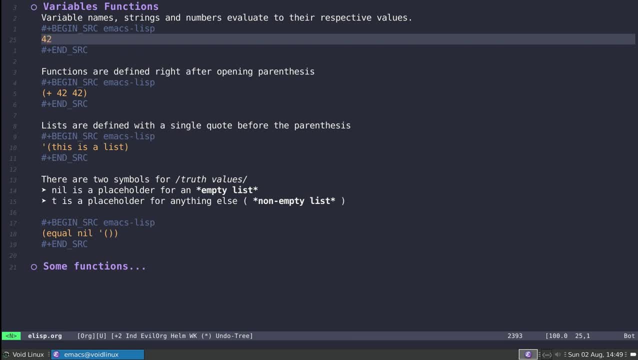 and numbers as usual. so 42, in this context, is going to be a symbol, and this symbol evaluates, evaluating it, and I get the return value 42.. So, essentially, 42 is a symbol, as I was saying, and I can also do the same thing for strings. So, for example, this is a string, Strings they are. 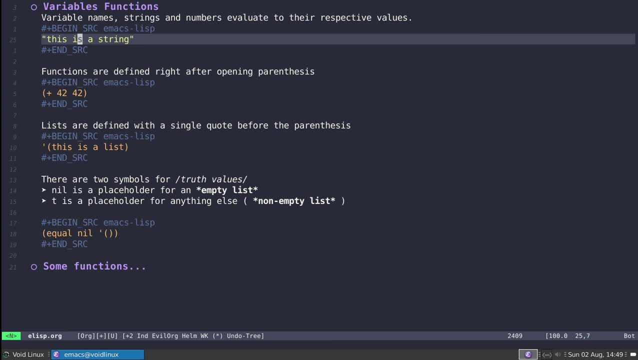 defined just as they are in other languages. so by using the double quotes and then ctrl c, ctrl c, notice that I get the return value. this is a string And I can also call variables. so in fact, let's say that I happen to know from reading the manual that there is this one variable built into. 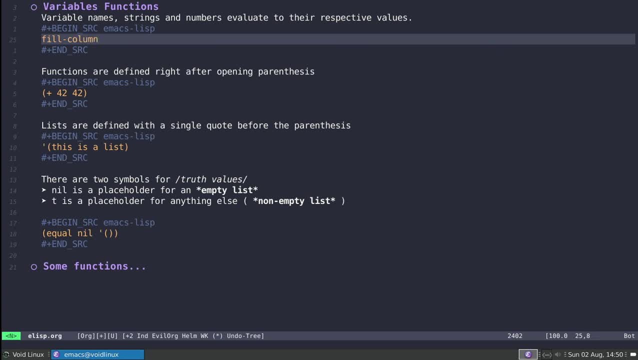 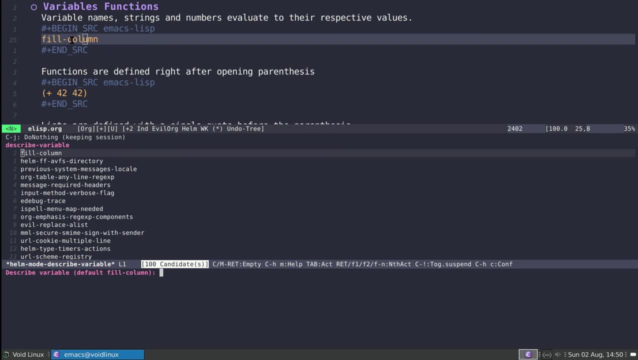 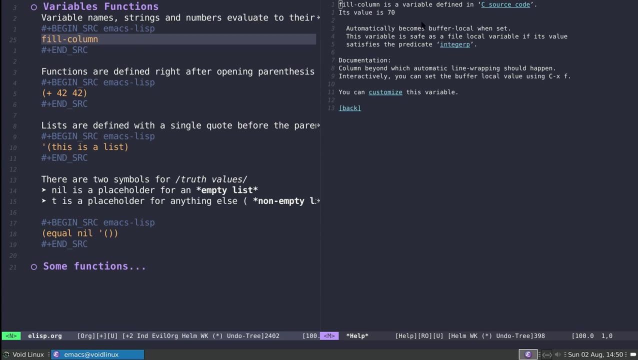 Emacs, which is called fill column, and if you want documentation on any variable, you always have the command ctrl h and then v, and notice that again since I, since on top of the word I actually get suggested the word itself. so I'll go with fill column as the as the description, and this is again. 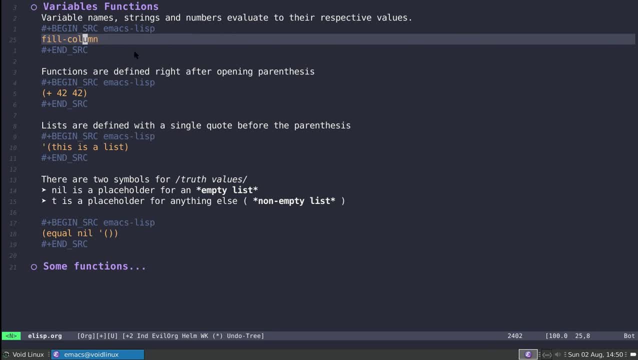 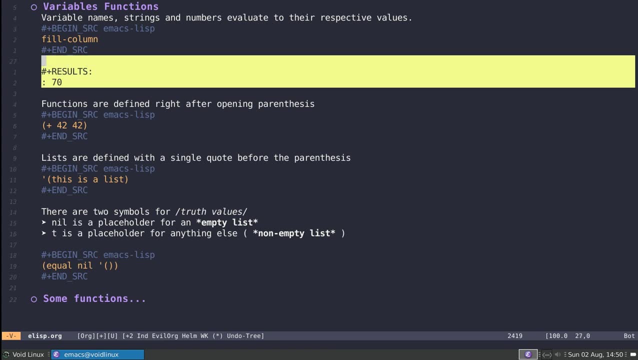 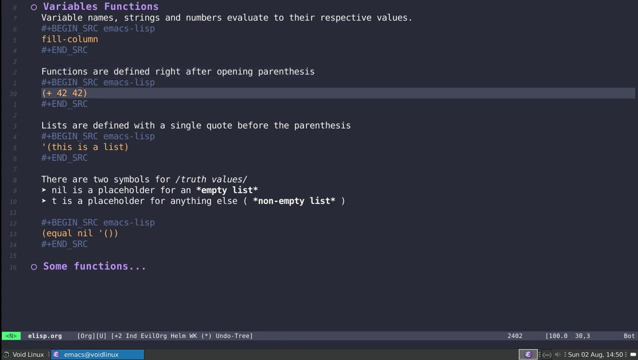 kind of a documentation on the variable, if you're interested. Now let's say that I execute this. I actually get back seven Because it happens that the fill column variable on my Emacs is equal to 70. And Lisp also has functions, and functions they are kind of the main part of Lisp, because Lisp 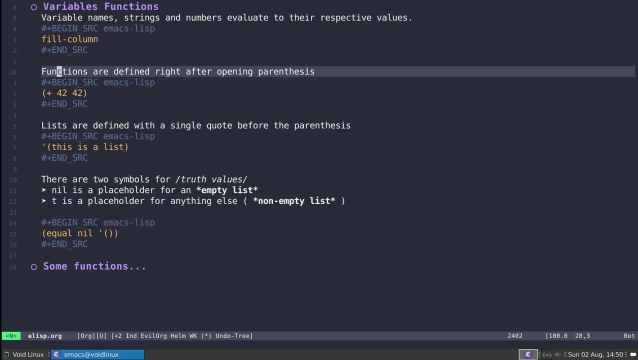 itself is a is a functional programming language and really a lot of the kind of behavior relies on functions doing things. So you're not going to see classes, you're not going to be to see object-oriented programming. everything relies on a kind of a functions and the functions they are. 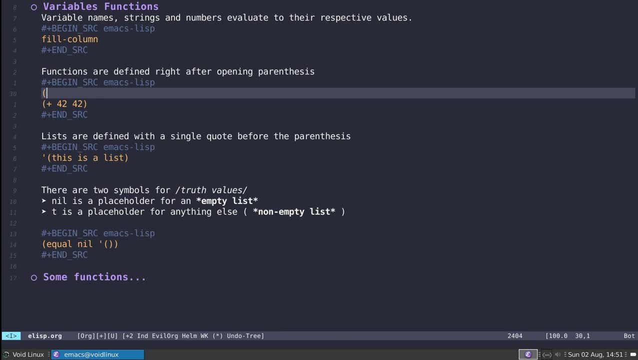 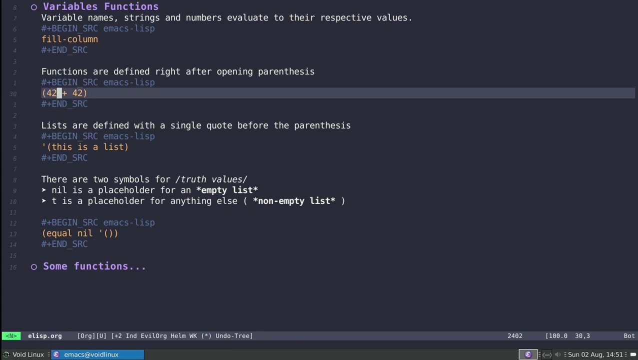 different. So I'm going to define whenever you open a parenthesis. so if I were to start opening a parenthesis here and then I write in something, for example, anything, so if I let's just say that the first thing that I'll do is I'll try to use an invalid function. so let's say that I want to sum two numbers. so this would be the incorrect way of summing two numbers, in fact, because essentially, the first thing on the parentheses is going to be the function and then you give it arguments. so this is something that's anti-intuitive if you're used to other languages. 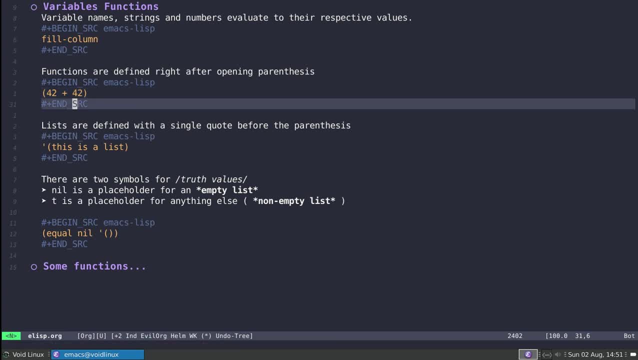 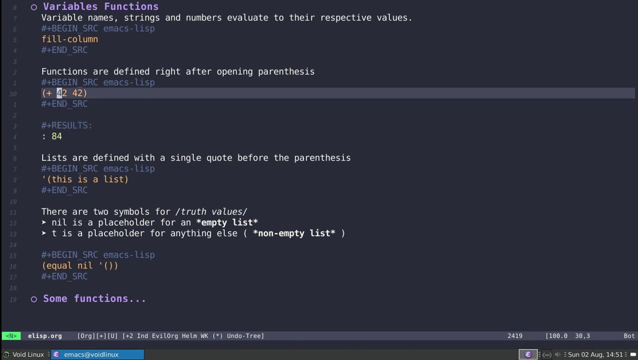 But this is how Lisp works. so if I try evaluating this, I actually get the response invalid function 42, because it's expecting the plus to be here, in fact to be on the beginning. but if I do it like this, I can execute this and you notice that I get the output 84, which is 42 plus 42.. 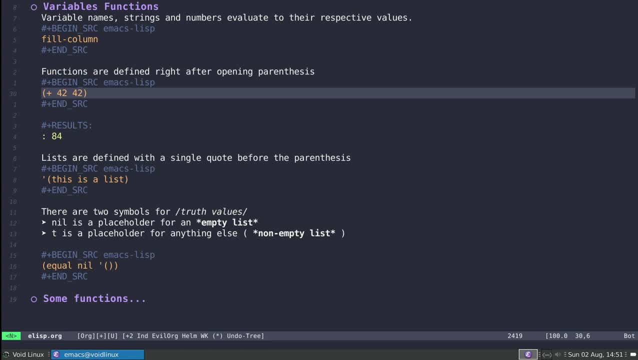 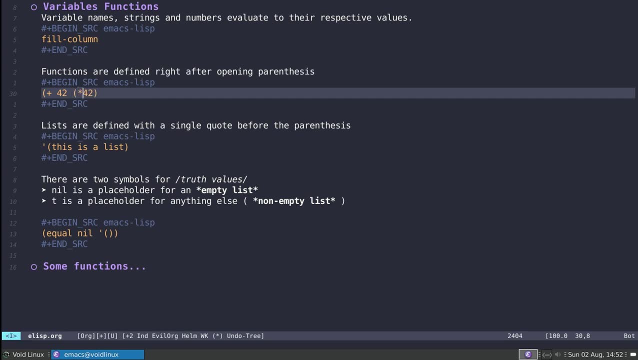 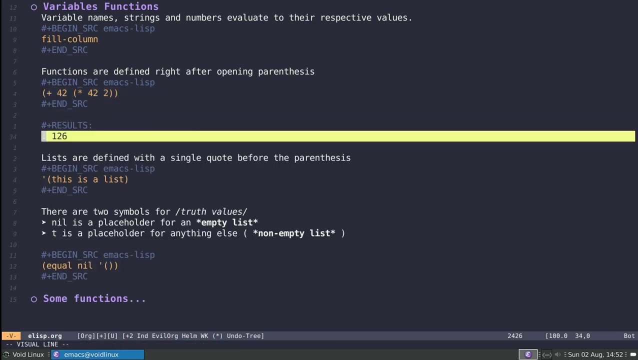 Now I can mix and match functions and I can also give the return of other functions to the two functions. so, for example, if I wanted, I could also make 42 times 2 and then sum this with 42. so the Lisp reader, it's very intelligent in that it parses the list accordingly and it knows that it needs to evaluate this part of the code first, and then it evaluates this part of the code first and then it evaluates the whole thing. so if I run that, I get 126, which supposedly is also 42 times 3. so because 42 plus 42 plus 42. 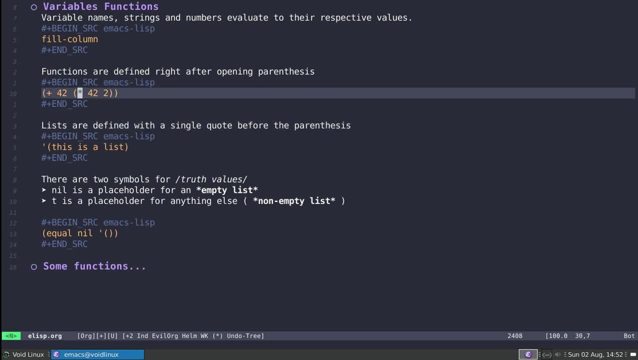 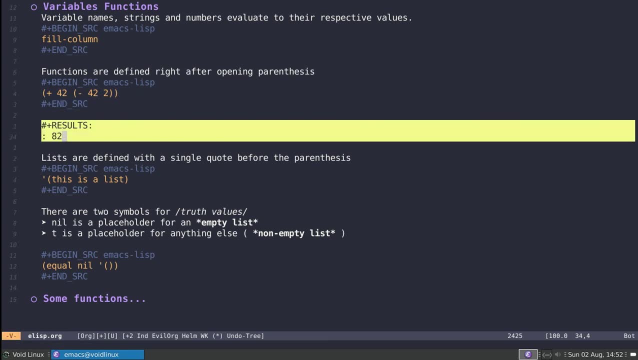 And again so mathematical functions. they are very simple. you have plus and you have times. you have minus also. so 42 minus 2 plus 42 is going to be 82, and you can also divide. so 42 divided by 2 is going to be 21, and then plus 32, and then plus 42, you get 63. 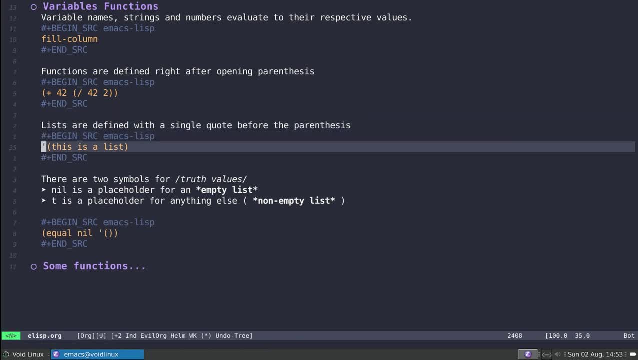 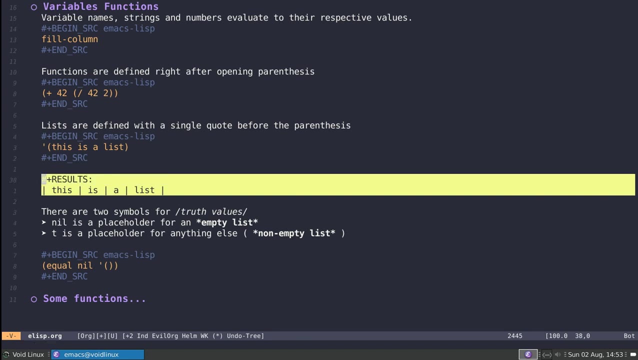 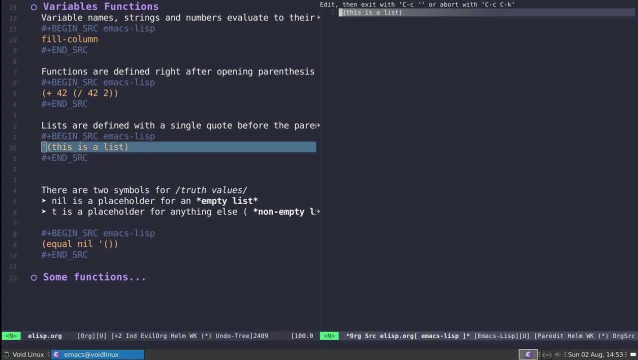 You can also define lists in Emacs, Lisp, and the difference is that you also use the parentheses but you can't quote the parentheses, And there are two syntaxes for that. so if I execute this, I actually get returned a list and org mode. in this case, it kind of displays the list as if it were the row of a table. just know that this is represented inside of Emacs. I can even open this on a Elist buffer. this is represented like this by using the parentheses. so this is a list. 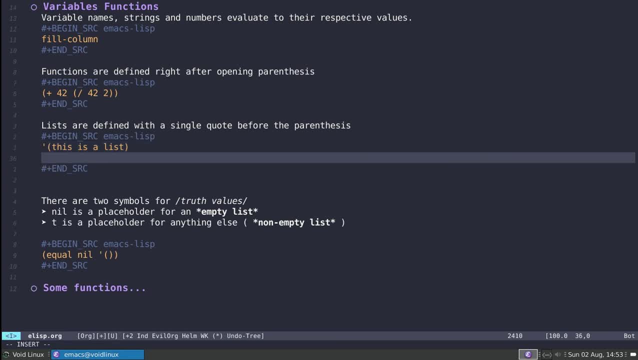 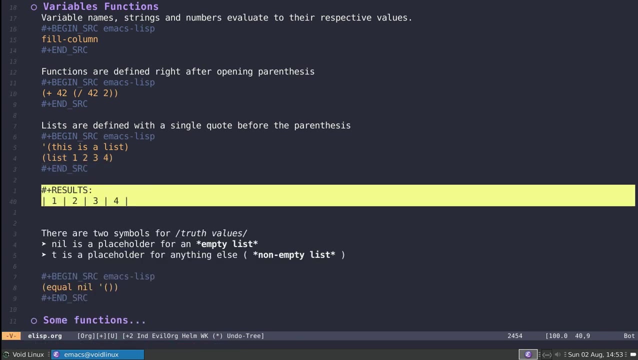 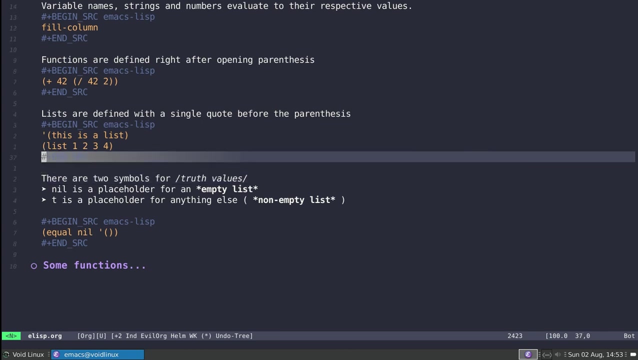 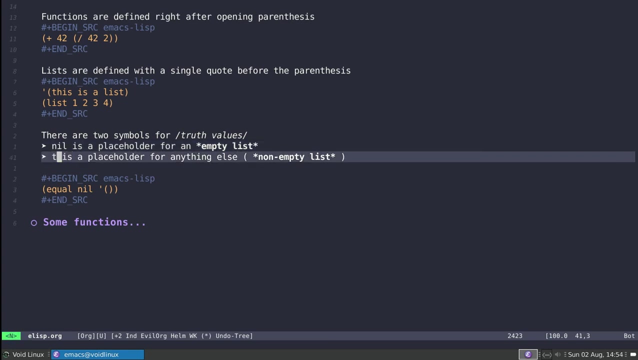 And there this is one of the ways you can also define lists by using the list Function. so if I write in list and then I give, and then I give it arguments 1, 2, 3, 4, for example, I can then execute this piece of code and I get returned again a list which contains the items 1, 2, 3, 4. you can also talk about truth values. so there are two kind of truth values in Emacs Lisp and they are nil and t. so these are kind of the equivalent, the analogous. rather, they are the analogous. 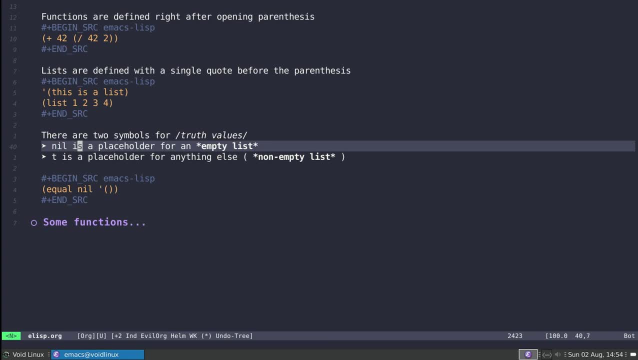 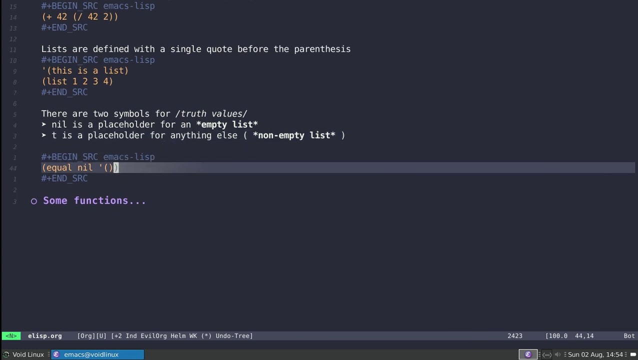 Versions of true and false. so new, in fact, is a placeholder for an empty list, so anything that's not an empty list is going to be considered to have a truth value of true, in fact. so these are placeholder for anything that's not an empty list, and I can even check this by using this little function which is called equal, and equal is a function that essentially compares things and it tells us if they're weak, equal and if they are the same type. so if I run this, 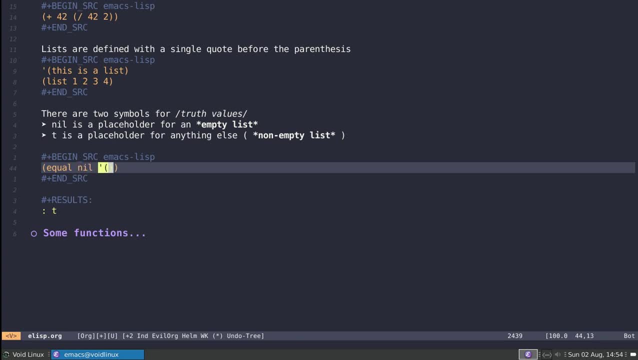 Notice that is nil. is nil equal to an empty list? and the result is yes. is t or true equal to an empty list? I'm going to receive nothing because by default org mode does not print kind of nil. so if I go to my again, to my e-list buffer, I can press control x, control e and you notice that I get nil as an output, because true is not equal to an empty list. 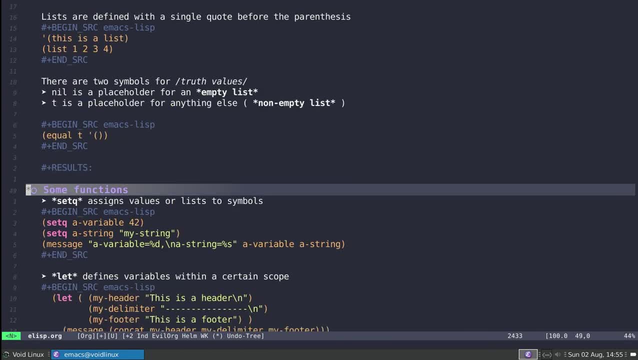 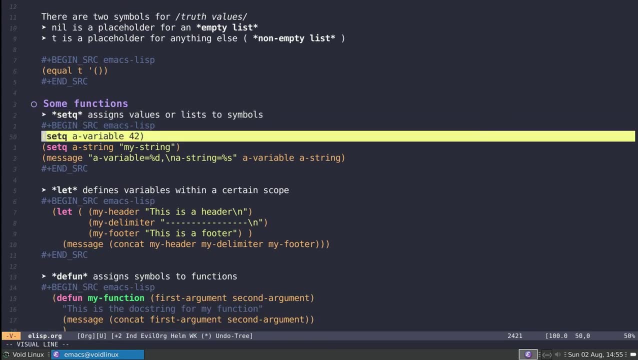 You also have some fancy Functions when it comes to this. so one of the most important is set q, and this allows you to kind of set variables. so, as an example, here I'm using set q and I'm setting it to a variable, to be the integer 42, and here I'm setting a string. so, again, a string is equal to the string. so the first thing, the first item, is always going to be the symbol that you're attaching the kind of the value to, and this is the value we call these symbols, by the way. so 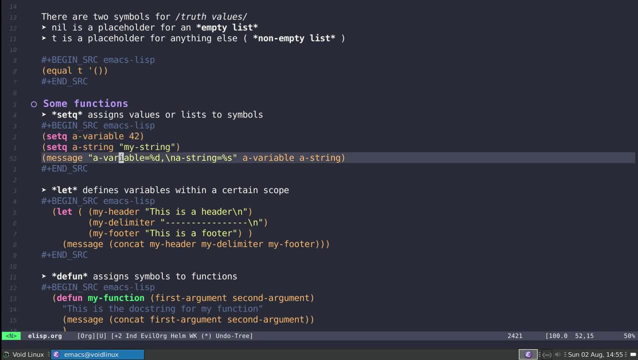 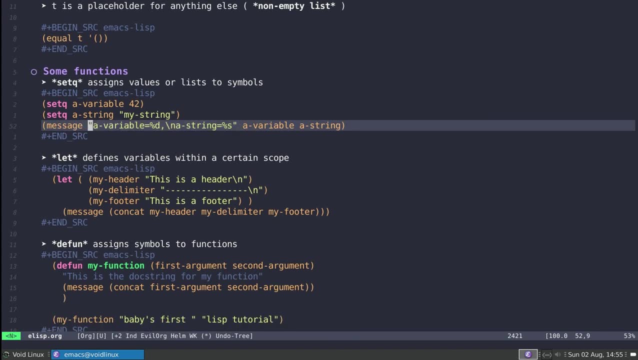 These Names that we give to stuff. they are symbols And I can use the message function in order to print that, as we were talking earlier, and the message is very nice because it works kind of like a. they print f function in c, so you can give it kind of this: a, this placeholder, this is a placeholder for an integer, the percent d. 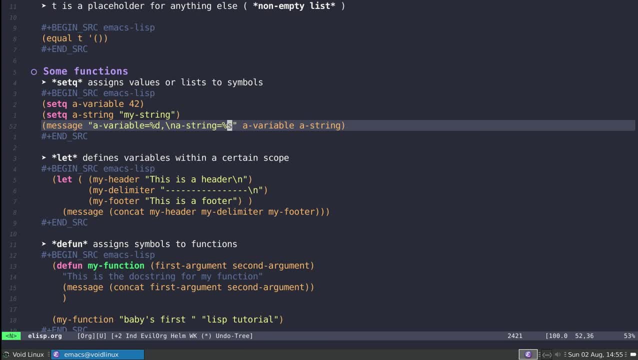 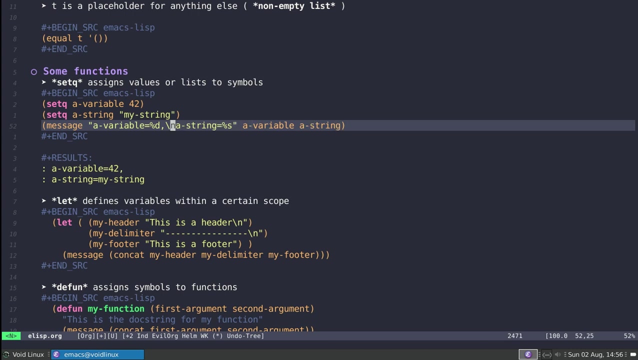 And this is a placeholder for a string. so this is actually the same syntax that you was on a format statement, for example, and then you give it kind of the Art Arguments that you put placeholders for. so I put a placeholder for the integer first, so I'm giving a variable, and then I put a placeholder for the string and then I give it a string. if I execute this, I get this nice output. you'll notice that I also have a little 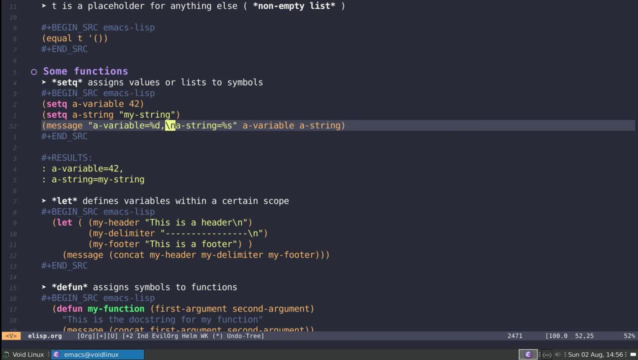 Backslash n and this is a jump to the next line. so this is why there is a jump from here to here And a variable. we go 42. my string equals to a string. so this is what set q does. it's essentially a science. 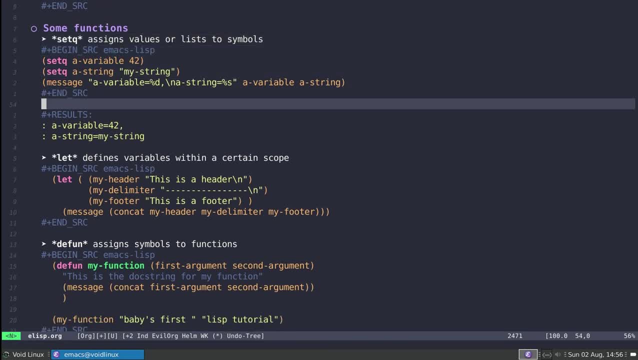 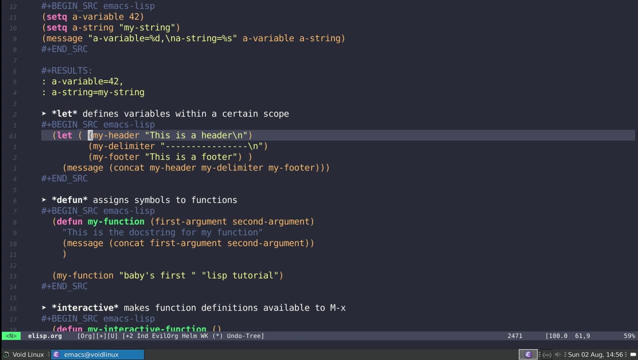 Values, values or lists to symbols. I also have left and let, this kind of a nice statement that essentially defines the scope within which a variable is defined. so in this case I'm using left and I do need this kind of outer, outer parentheses, and then inside of it I can give these kind of lists in pairs. so this one is going to. this part is going to assign my header to the value. this is a header. 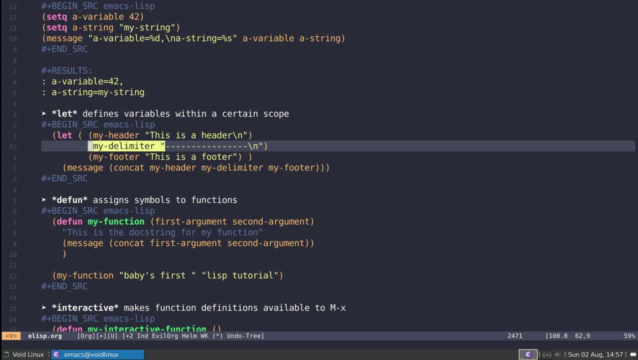 And then my delimiter is going to be a sign that this kind of string And my footer is going to be assigned. this is my food and this is my food And inside of this let statement these three variables. they are defined and I can use them, for example, on the message statement. and then the message statement it's using the com cat function, which stands for concatenate. so if I give it a number of strings, it essentially is going to concatenate them one after another. 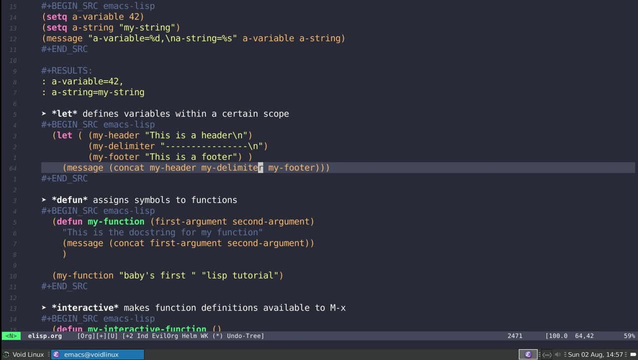 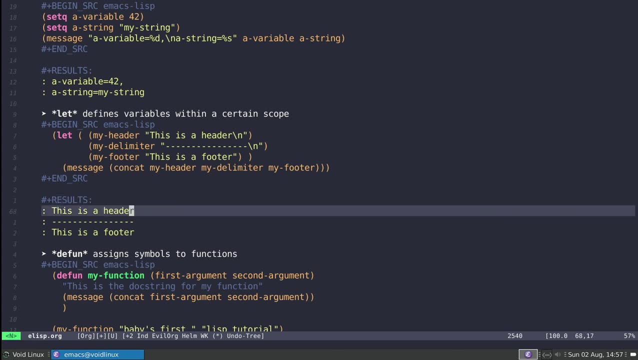 And if I try this, So I'm putting all of my three variables in order- I can execute this code and you notice that I get the output. so this is a header. and then I jumped next line and then I print my delimiter. and then I jumped to the next line and then they print my foot. 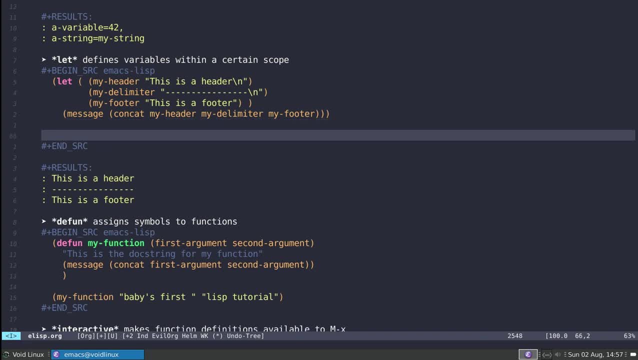 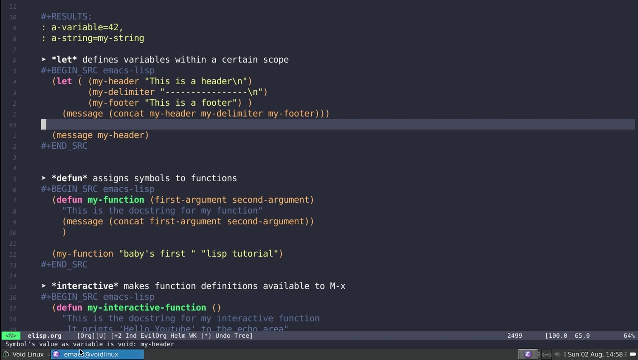 If I were to try to use these variables outside of the let statement, they will not. they will not be defined. so I can even try that I can use message my header, just so that I can print: this is a header And let's see if that works. so if I execute this again, you notice symbols. that symbols value as variable is void because again, I am outside of the scope of this variable. so the list compiler, the list or reader, does not understand that this variable is defined out here. 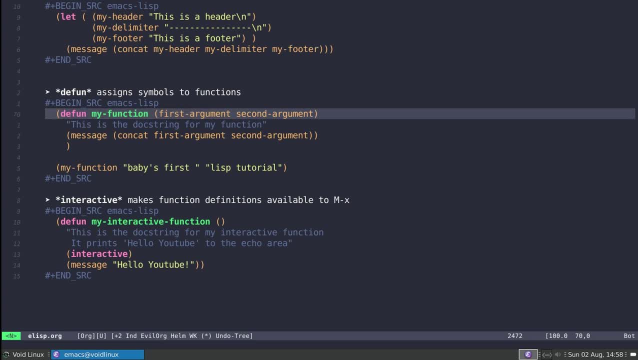 You can also define functions by using this kind of defun function, and the syntax is very simple. so you define the function name again that you're at, this is the function symbol- And Then you give it a list of arguments inside of this kind of this kind of parentheses. so here I have a first argument. 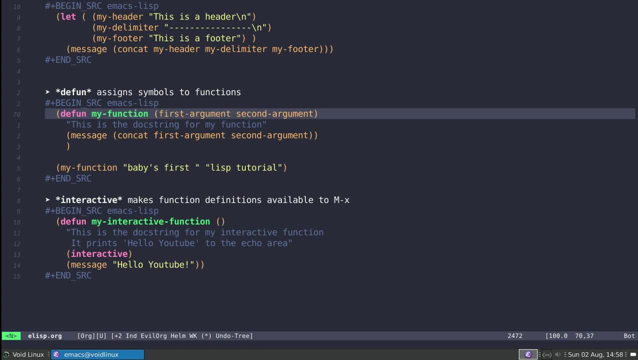 And you notice that we usually kind of separate things using dashes. so this is the most, I would say, the most- used way and this is the best practice also. So we also have a second argument and usually function definitions. they come with this syntax and I can also write doc string, so whichever string I write, 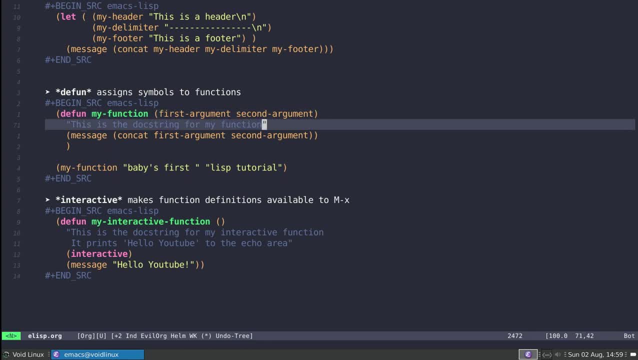 I write right after the, this kind of parentheses is going to become the doc string for my function, and the doc string is what appears in the manual. so in this sense he makes this this kind of self documenting, because whichever, whatever you write as a kind of commentary here- pseudo commentary anyway- is going to appear on the manual of the function directly. so you write code together with documentation. 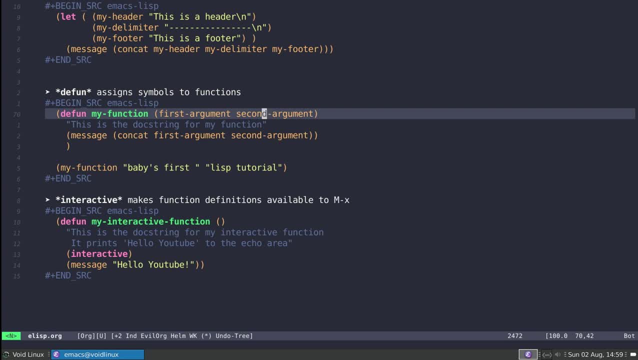 And in this case what this function does. so it defines the arguments, it defines the doc string and then the next time The next thing that you do is you essentially give it the instructions to evaluate. so in this case the instructions are: use the message function and then concatenate the first argument and the second argument. so in this case I'm supposing that the first argument in the second argument they are strings, because I can concatenate them and because I can print them and later I can call this function as I would any other function. so I open parentheses. 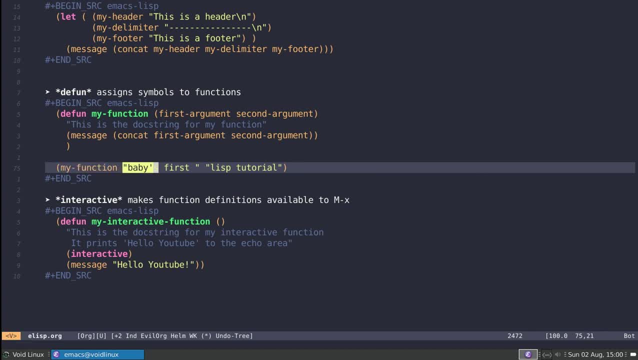 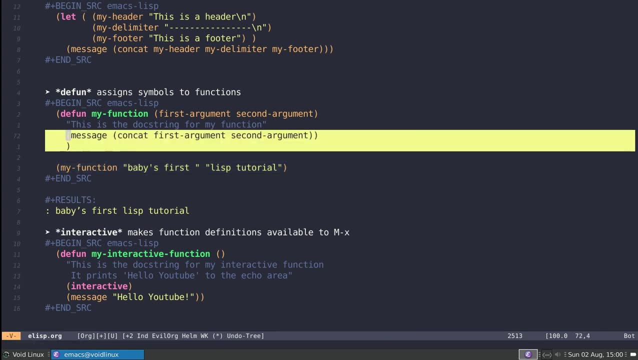 And then the first thing that I call is my function, and then I give it two strings. so this is the first argument And this is the second argument, and if I execute this, the function is defined and then I call it and this is what it outputs. so baby's first list tutorial. notice that it's concatenating. this is my first argument, and then it got concatenated with the second one and then got printed. 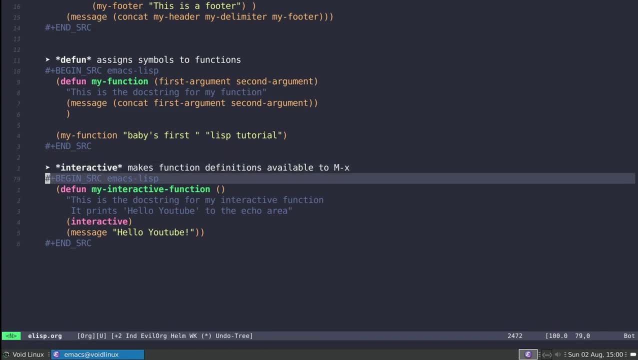 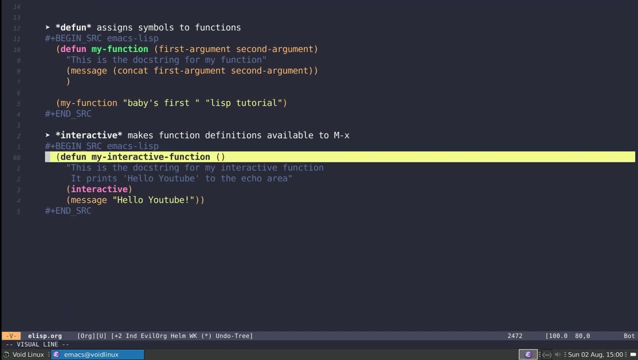 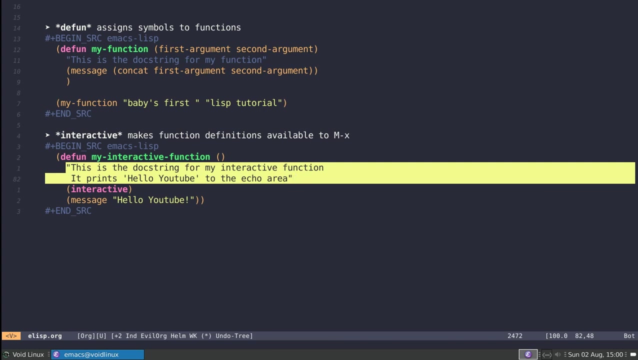 Finally, you have a nice function which is called interactive, and you can put it inside of your death, of your defined function statements. so, as an example, this is an interactive function And I define here a two liner to be my doc string. you notice that I just need to put my, that, my, my kind of documentation, inside of this little set of double quotes. and then what is important is that, right before starting my, my 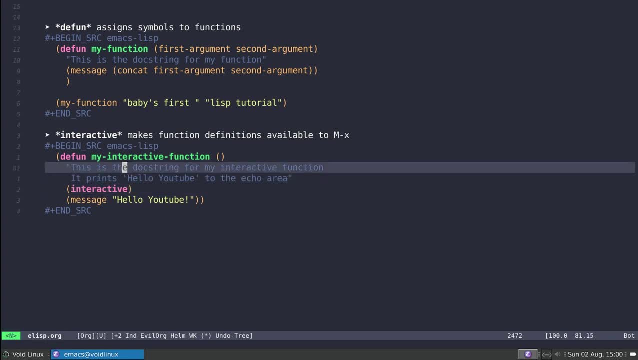 My expressions. I can then use the interactive keywords. notice that this time there is no, there are no arguments, so this function is going to be called interactively, which means that they essentially I can call it using a meta X, And so if I evaluate this as a return value, I get kind of the symbol that I am defining and now the function is callable from my e-mags, so you can press meta X. 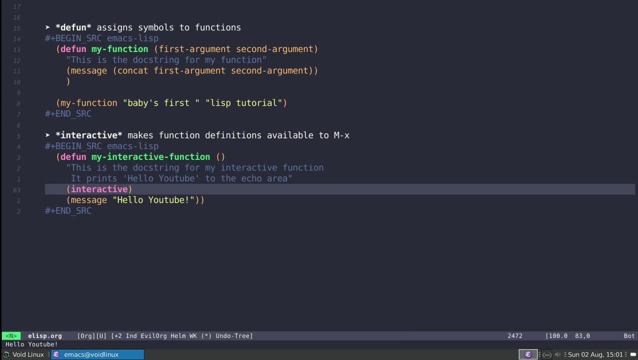 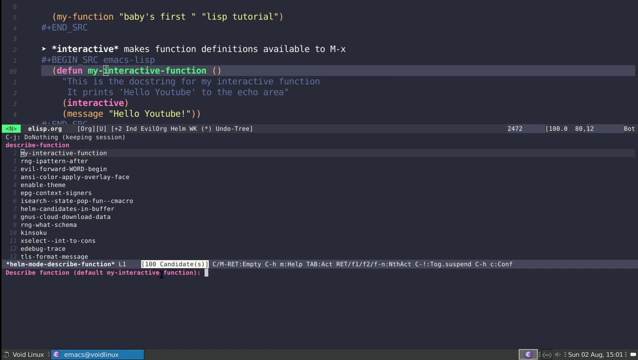 And then my interactive function. You notice that I get hello YouTube printed down here And additionally I can also refer to the documentation of it. so if I go over my interactive function and press control HF, You notice that my interactive function is available. 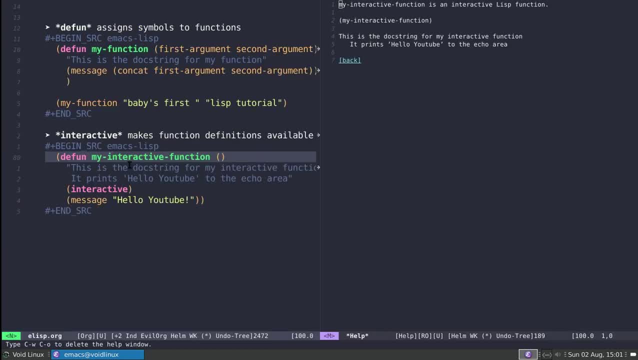 so in fact, the doc string that I defined here is what appears here on the manual. now this is, I think, a good, a good beginning in terms of lisp. we haven't touched on kind of control statements or anything else. we looked a bit how to kind of define variables and also how.